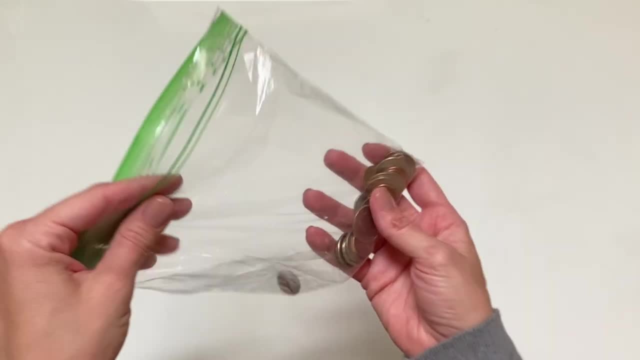 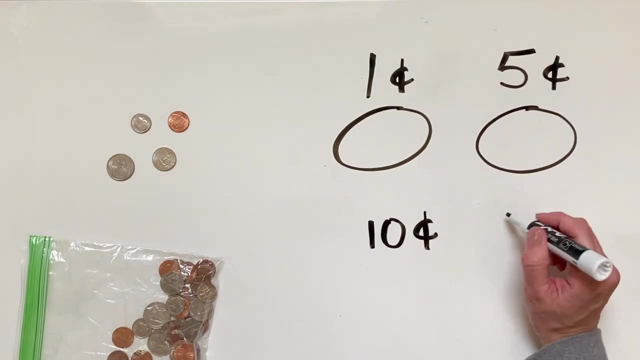 laying around your house. This is a little abacus that I found useful in my homeschooling. It's coins. Kindergarten and first grade is when kids start learning money concepts, especially cents. if you're in the States, I always found real coins and a whiteboard are a fun way to practice recognizing what the value. 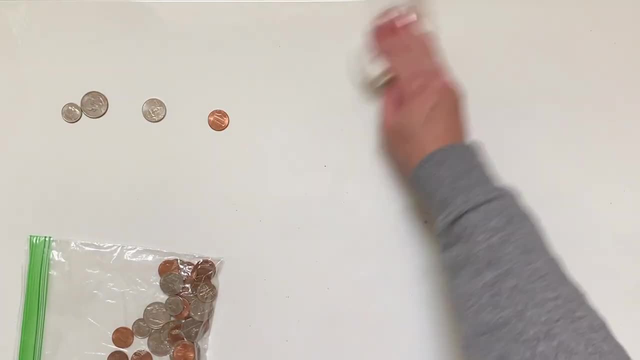 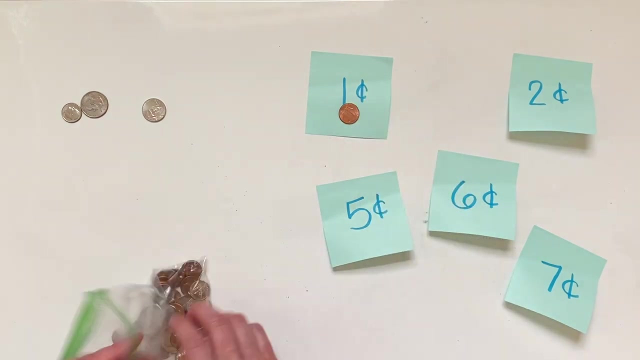 of each coin is. One popular game in our house is called store, where I write different amounts on sticky notes and create a store by sticking them on different toys or items around the house. Then I have her purchase these items by counting out the right amount of change. 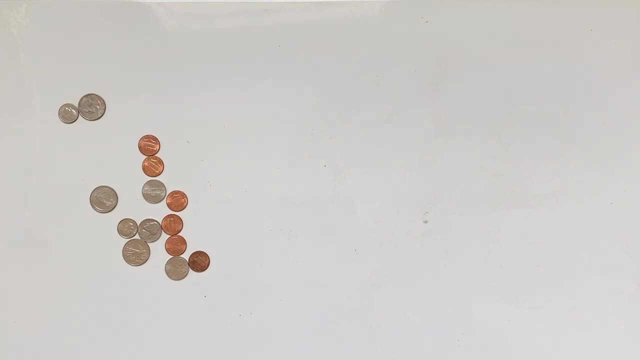 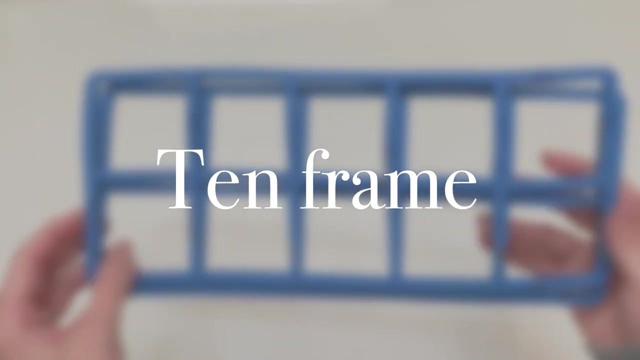 Coins have been a popular manipulative in our house and the best part is, like I said, they're already lying around the house or the car, so no need to purchase this one. Next up is the magnetic 10 frame I found on Amazon. A word of warning: these are not toddler. 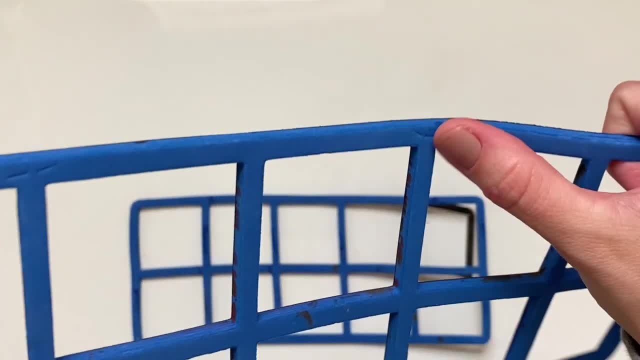 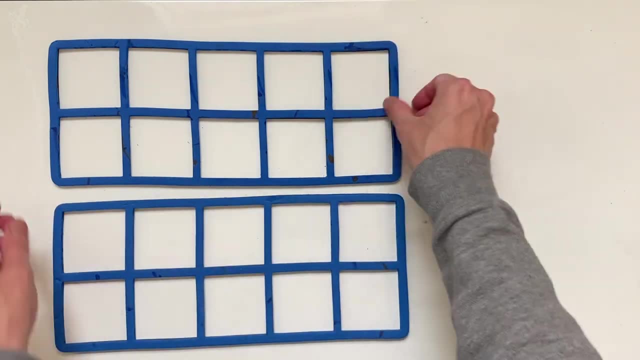 proof, As you can tell, ours has really taken a beating. Are those teeth marks. Anyways, I love, love, love that these are magnetic. We can just throw them up on the fridge or a metal whiteboard. I have let my kindergartner use markers to fill in the 10 frame, but they 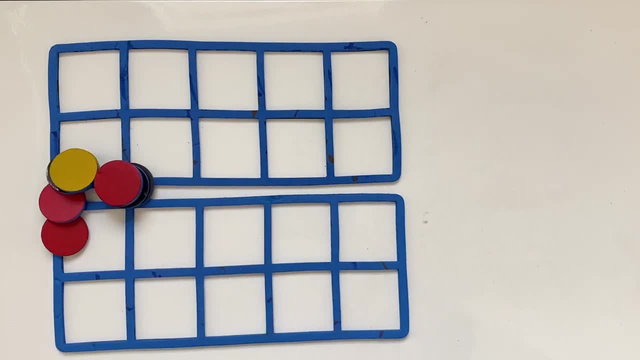 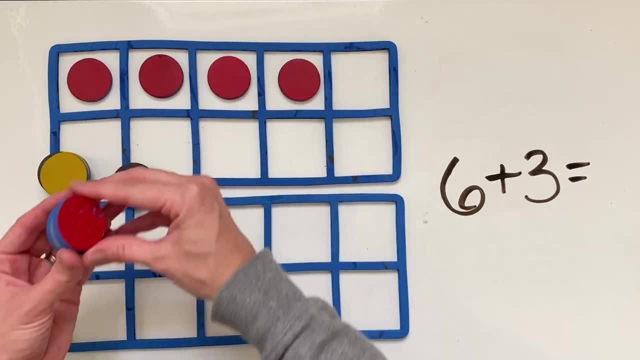 also come with magnetic dots: 10 yellow ones and 10 red ones. The 10 frame in general has been my absolute favorite way of teaching my daughter math, And having a physical one like this has been really fun for playing games or just quizzing her knowledge about addition. Yep, that's definitely a. 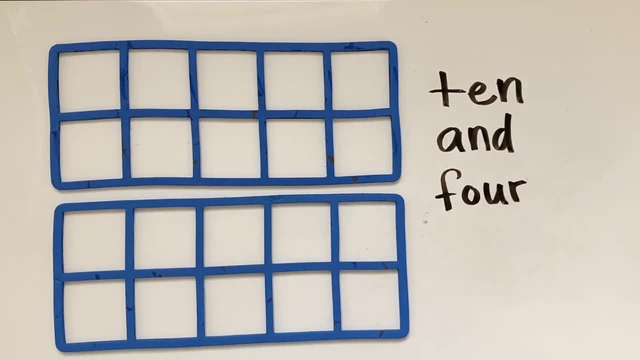 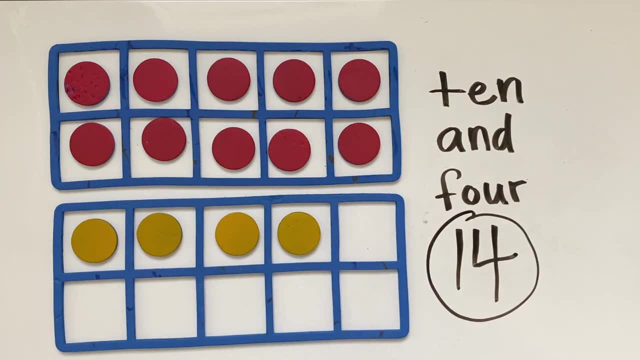 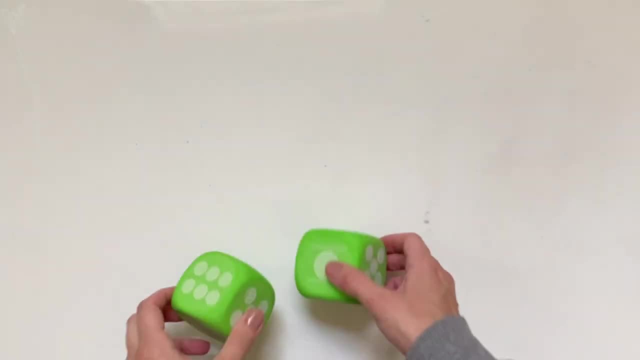 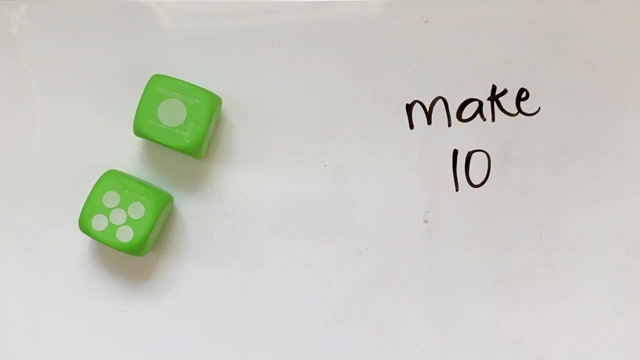 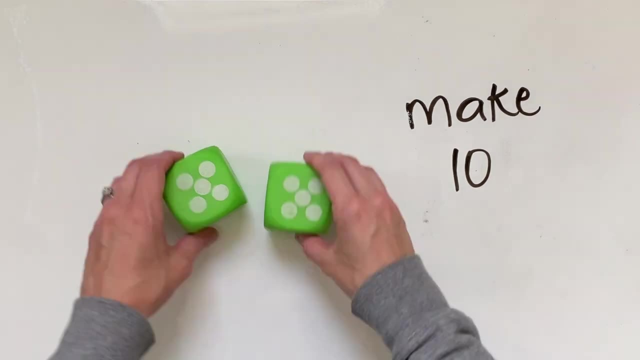 year round in the toy section. Again, lots and lots of addition practice with these. There are certain math games I have found online that require dice as well. It's helpful for little ones to be able to count the dots when adding numbers together. 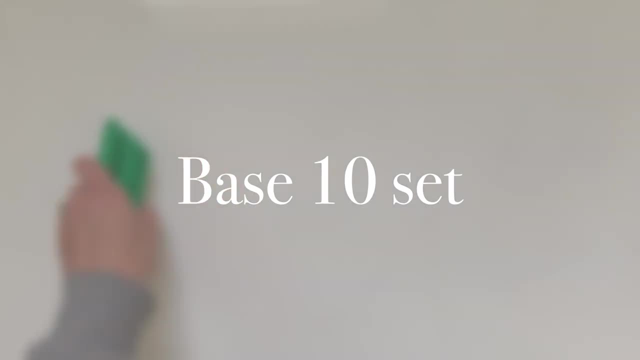 Next up is a base 10 set. This set originally came with the yellow ones units: 10 stacks of 10 in green, 10 100 flats in blue and a red 1000 cube. This set is a little different. 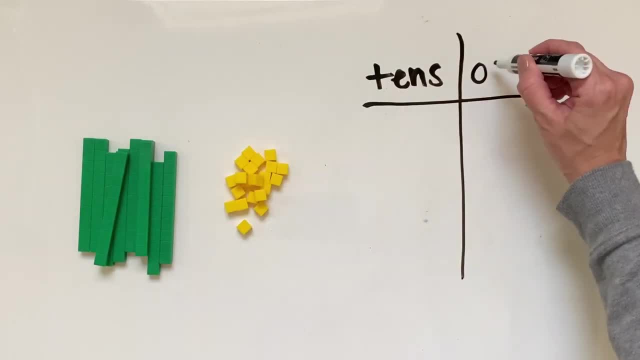 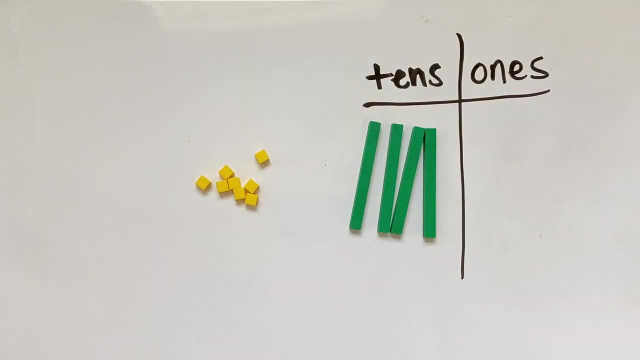 But for kindergarten I stuck with the ones and tens. A very obvious use for these manipulatives is place value practice. They provide a visual and tactile representation of numbers and groups of numbers. Some teachers and homeschoolers prefer when the tens can be taken apart and manipulated. 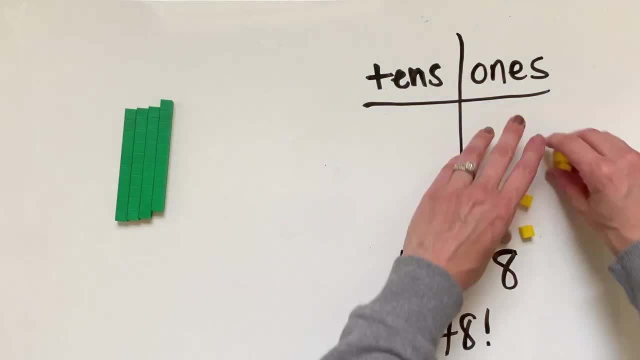 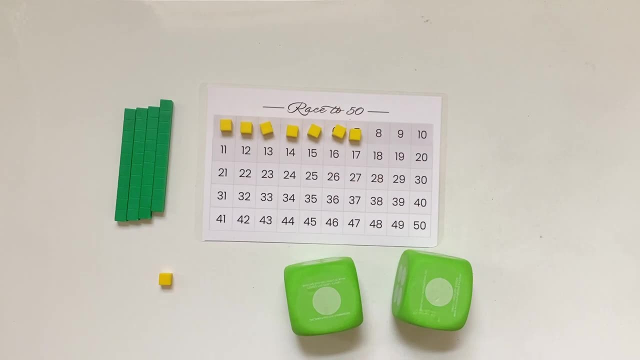 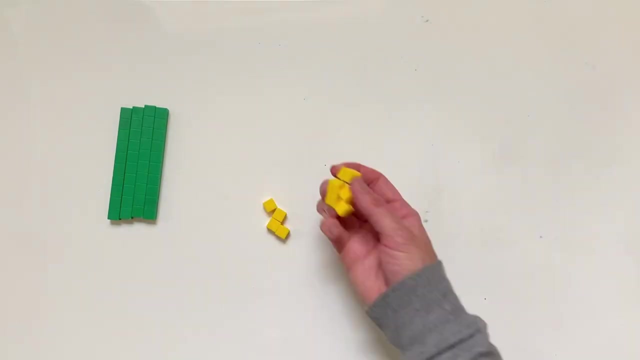 more that way. In that case, there are those popular stacking cubes you can purchase instead. I like to use these almost every week in a game called Roll to 50 or Roll to 100. It's a game that gets kids comfortable with the 100 chart and place value. 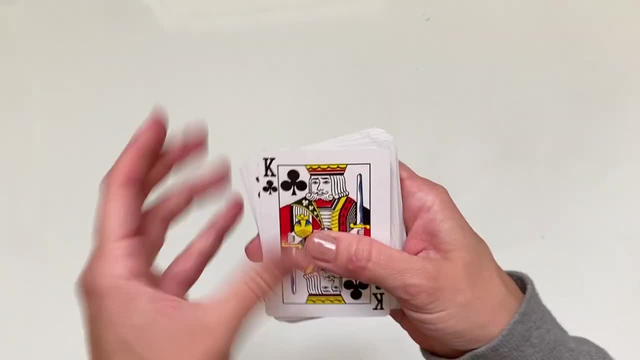 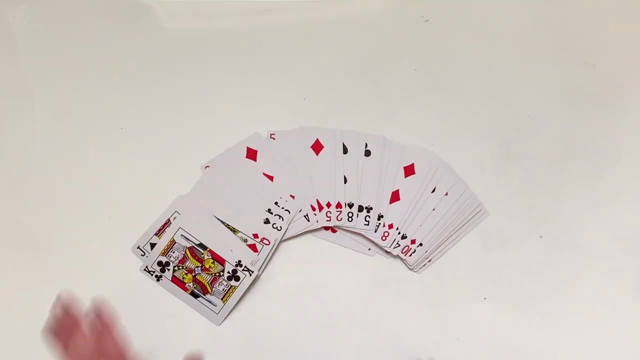 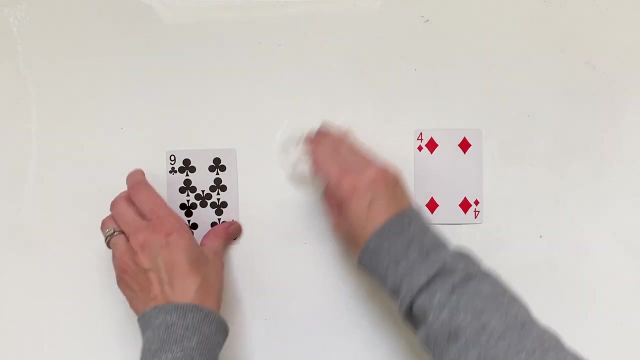 Another wonderful, extremely affordable math manipulative is a deck of cards. I'm not exaggerating when I say there are so so, so many uses for a deck of cards when it comes to teaching and practicing math. I'll use them to play little whiteboard games like greater than, less than and equal to. 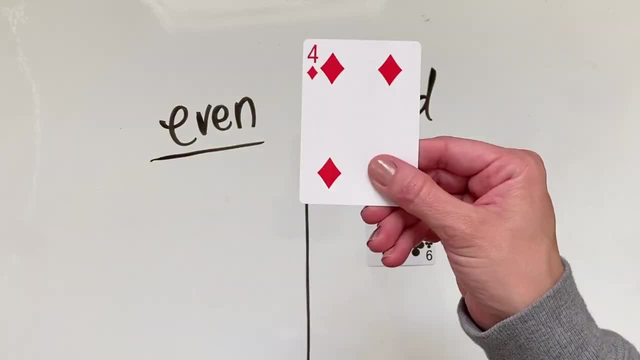 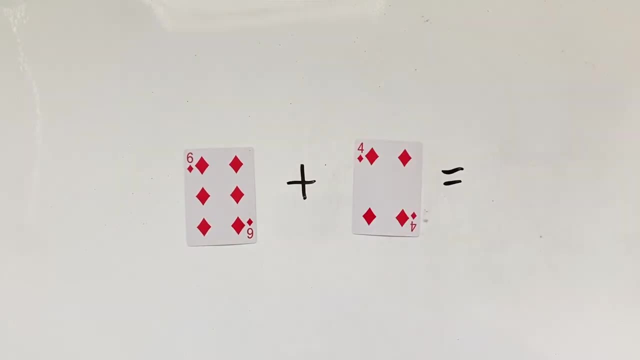 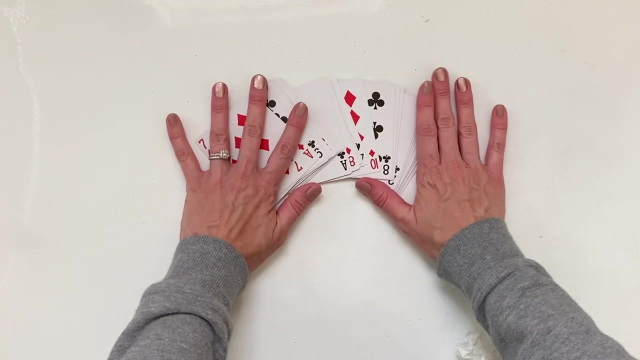 I use them to help her practice, Even in odd numbers. Of course we use them as addition practice as well. There are also so many card games out there that you can find with a quick Google search. Let me know if you would like me to make a video on different math card games I play. 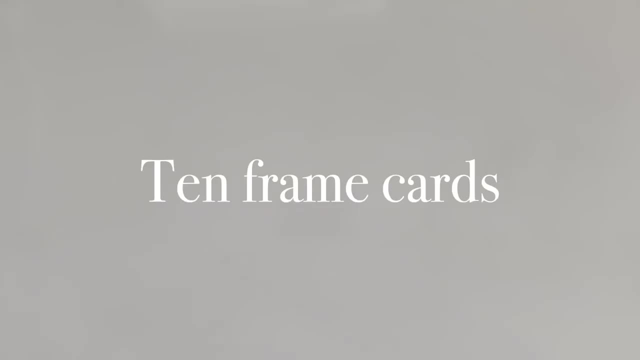 with my daughter on a weekly basis. Speaking of card games, I found these free 10 frame printable cards on Teachers- Pay Teachers. All you have to do is print, cut and if you want to get a little fancy, you can print it. 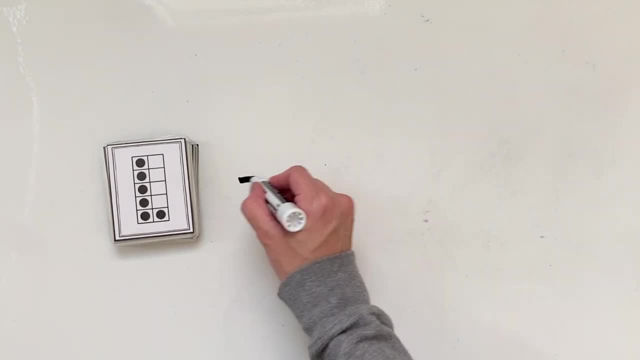 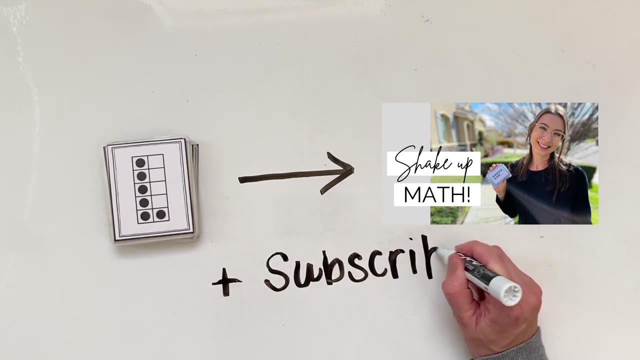 Or you can laminate them as well. I already made a video last week on what games we play with these cards and I'll link it in the description box below. And while you're at it, how about you hit that subscribe button so you don't miss all? 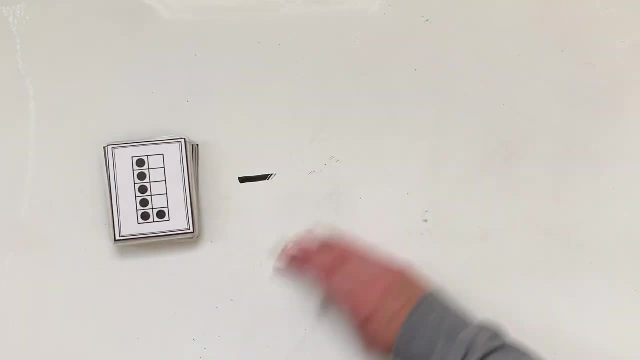 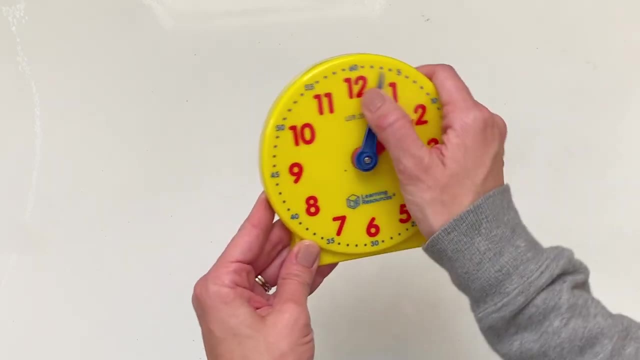 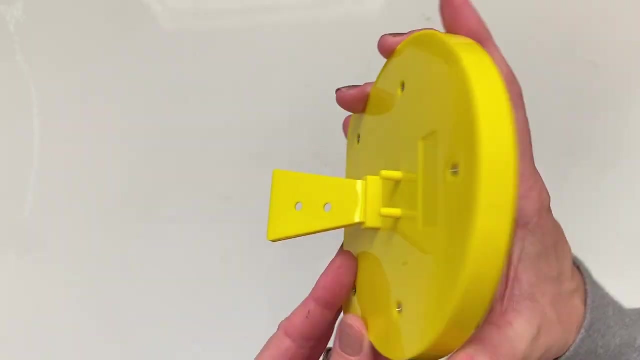 of the learning content that's coming up. This clock manipulative is probably the most popular one out there, and it's for good reason. The student can literally manipulate the minute and hour hands when learning how to tell time. It also comes with a little stand so your child can stand it up if they wish. 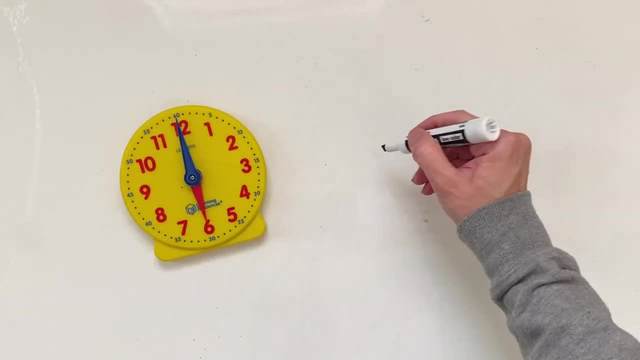 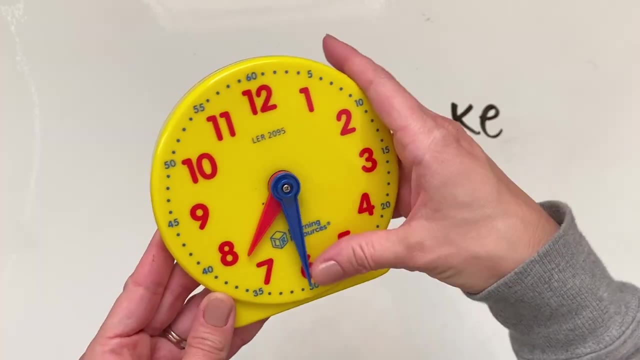 The obvious uses with this one is to learn time. I'll usually quiz her knowledge by adjusting the clock and having her tell me what time it says and having her write it down, Or vice versa, writing a time and having her adjust the clock.